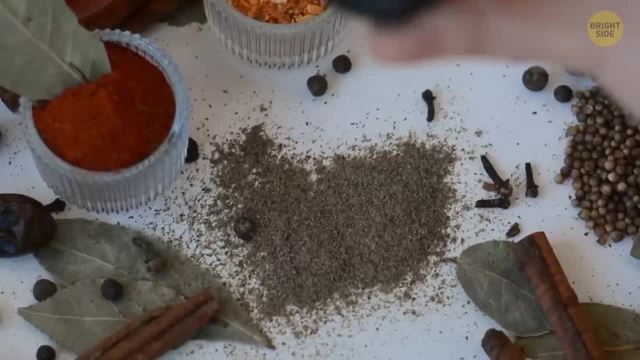 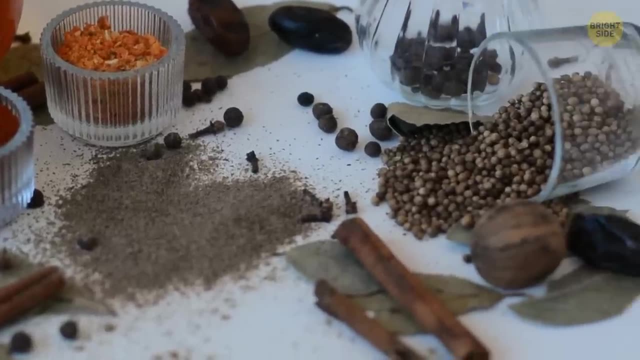 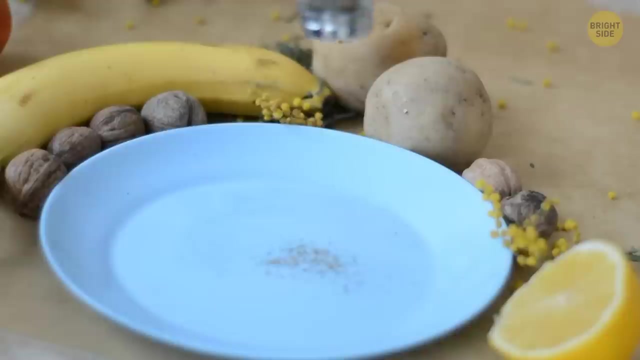 Now gently twist the bottle from side to side and before you know it, you get some gorgeously flowing seasoning without having to wiggle the shaker and make a mess all over the stove. On the same note, most salt and pepper shakers should have ridges on the bottom of the glass portion. 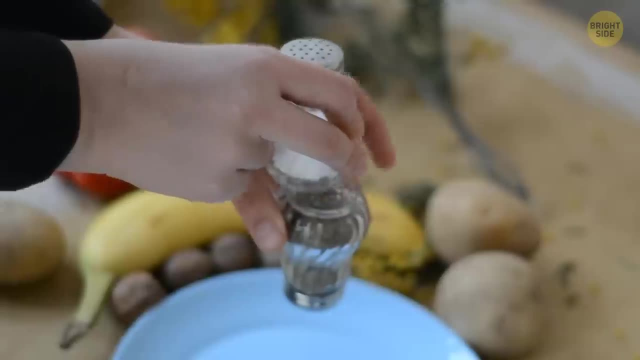 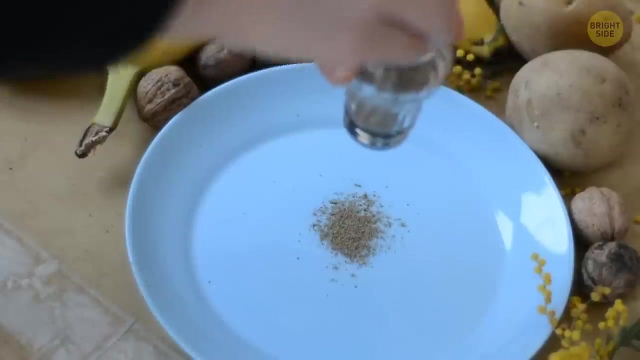 In case you get any seasoning stuck in there, place the bottom of the salt shaker against the bottom of the pepper shaker and wiggle it around so the ridges click with each other. The seasoning should easily pour out now without you having to open the bottle. 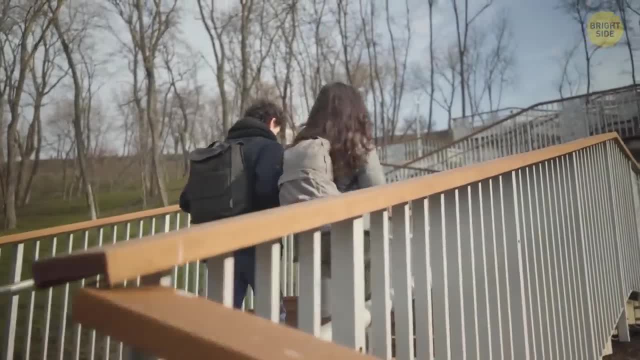 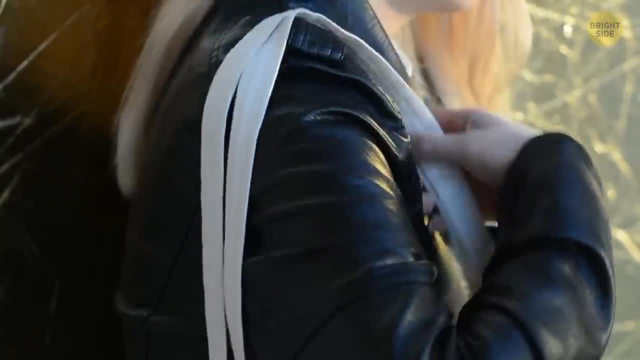 In colder weather, you often have so many clothing layers on you that you can hardly feel the purse or back straps on your shoulder anymore, Not to mention how fast they can slide off. Some jackets come with a built-in solution for that in the form of a small tab on the shoulder. 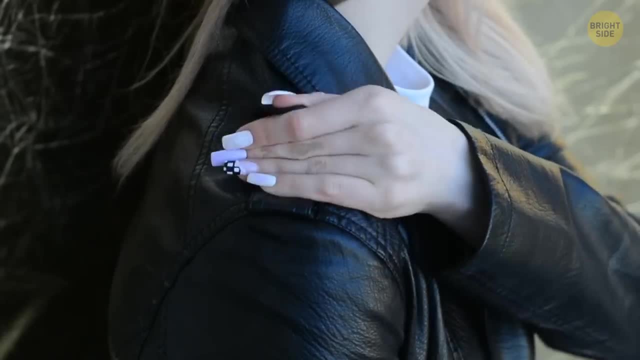 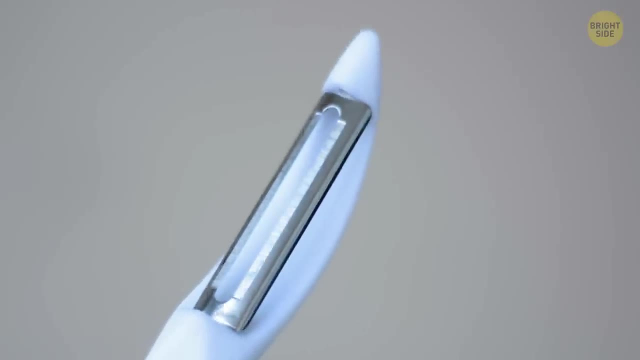 with either a hook or a button. It's meant to be open and then closed comfortably so you can keep your purse in place at any time. You're most likely using it merely to peel the skin of potatoes, carrots or cucumbers. 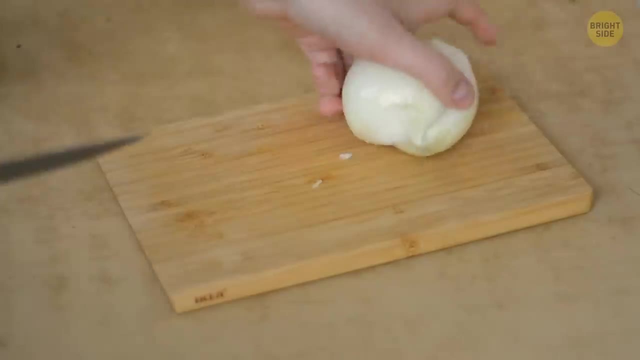 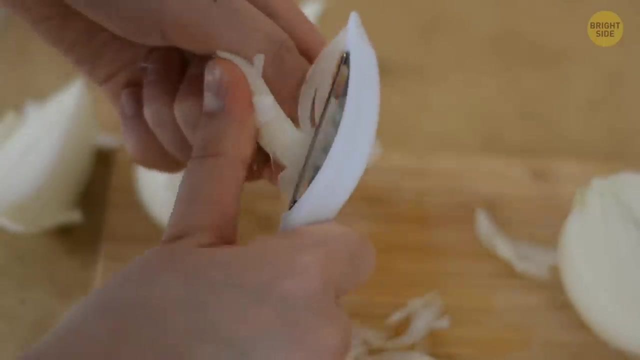 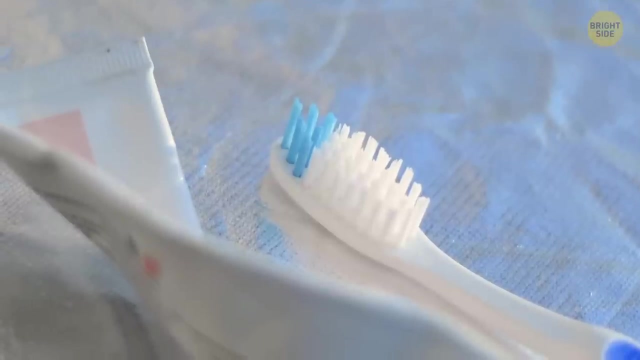 But you can use your vegetable peeler for chopping fine strips of onion as well. Just cut the onion into quarters vertically and then start slicing. This might also help out with those embarrassing onion tears. Most people miss this one, but should you ever have a closer look at your toothpaste? 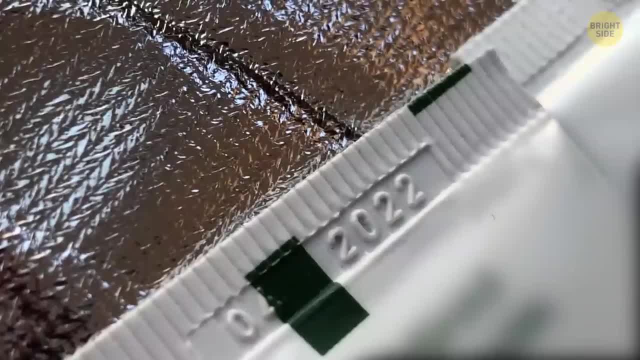 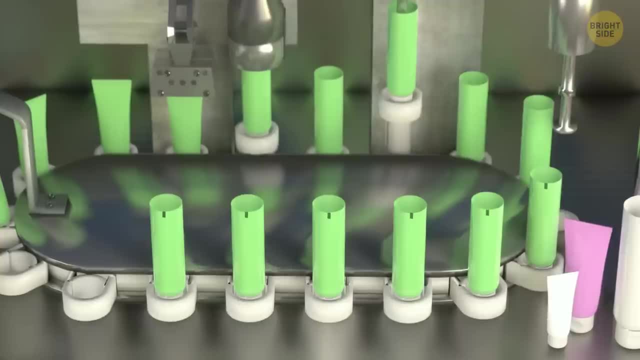 you will surely see some sort of coloring there, Either a dot or a block. Colors can vary. They can be black, green, red or even blue. These color spots are actually meant to help the assembly machines back at the toothpaste factory. 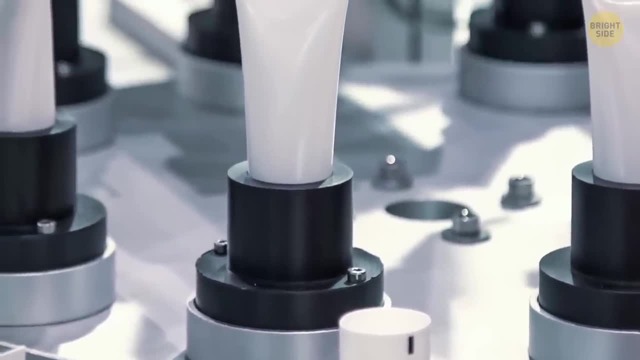 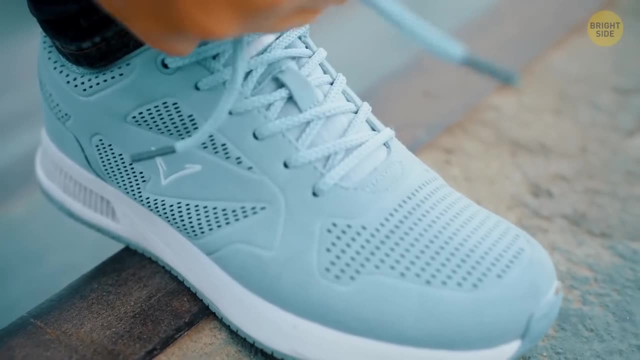 They recognize when and where these machines need to cut the toothpaste tubes and proceed to fold them for packaging For most types of footwear. if there's anything that seems a bit out of place, always know that it's there. for a reason. Most manufacturers don't put extra items on shoes just for fun. 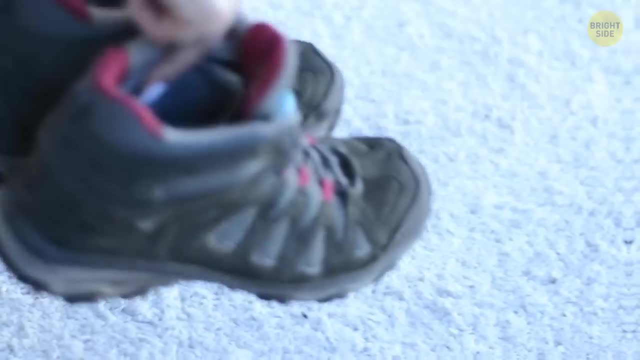 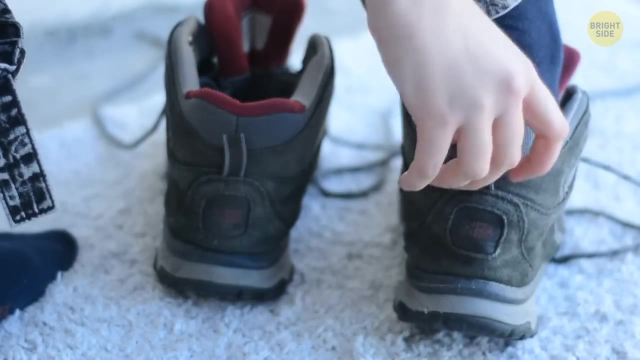 It would definitely be a waste of time and resources. For footwear like boots, for example, there's often a small loop at the top back of the shoe. It's there to help you when you need to put the shoe on, since you can quickly pull on it. 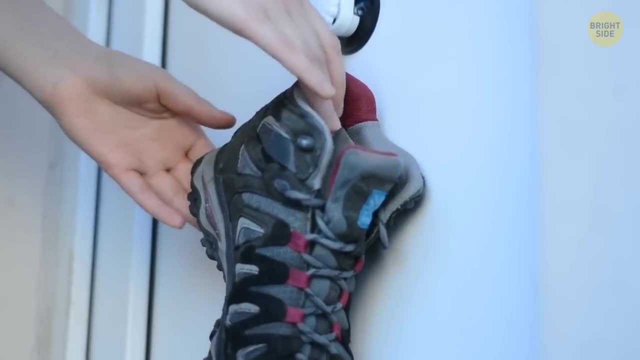 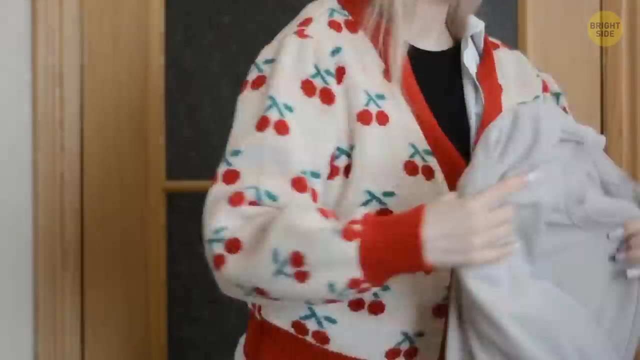 Plus, you can also hang the shoes somewhere most likely to dry, since most boots are meant to be worn in the colder weather. Now I've been guilty at least once of overdressing with a bunch of layers, just so I won't need to jam everything in my check-in bag. 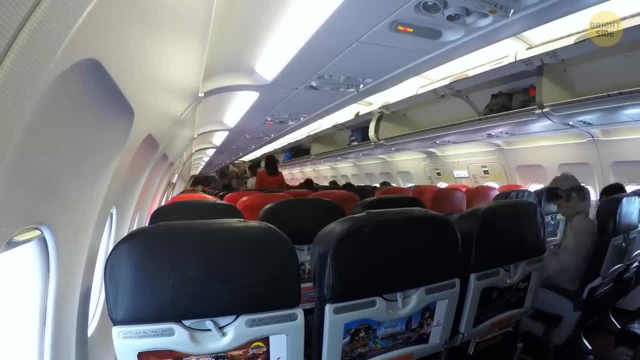 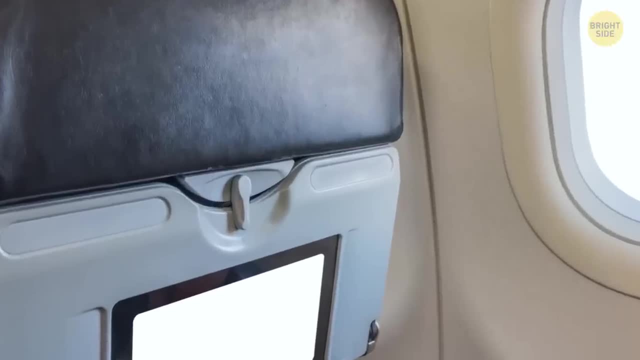 But does it become a problem when you actually have to get seated? What do you do with your coat or your jacket? Well, have a closer look next time you board a plane. on the seat in front of you, The hook that keeps the tray table upright. 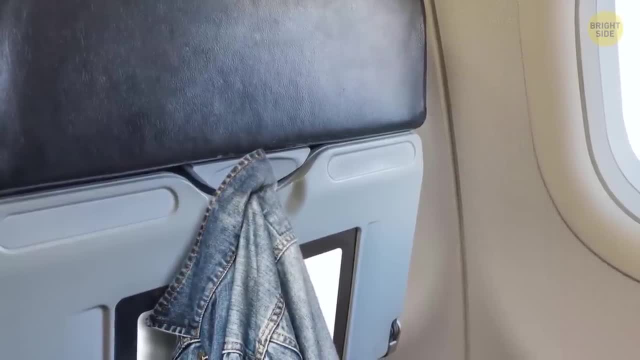 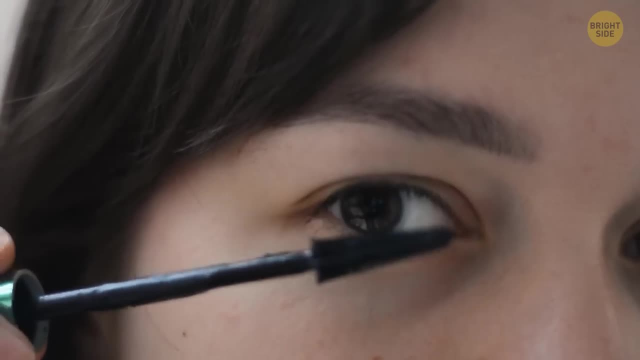 can double as a jacket hook. As long as you don't need to have any meals while in the air, you're good to go Now. most mascaras expire within 3-6 months, I'm told, depending on the manufacturer. 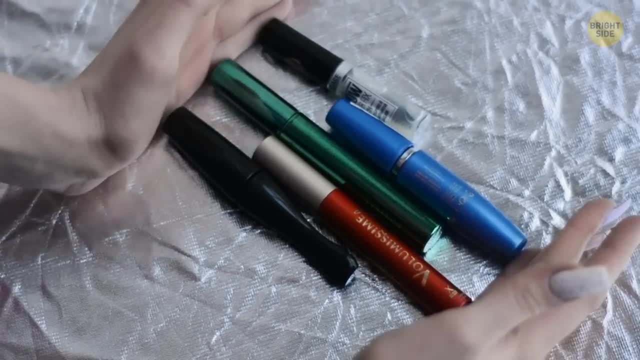 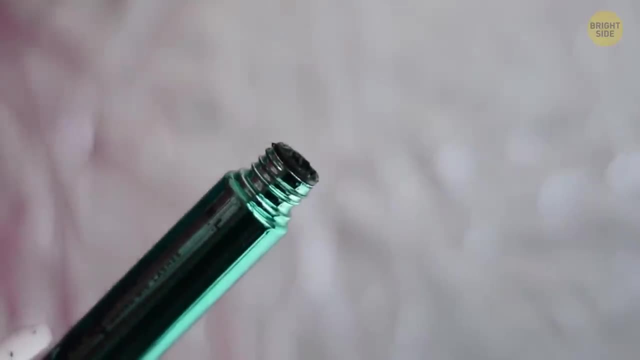 But you can help speed up that process. if you're not careful enough, Continuously pumping the mascara wand trying to mix in the product actually pushes more air into the tube. This can make it dry much faster and you evidently won't get the desired results with it anymore. 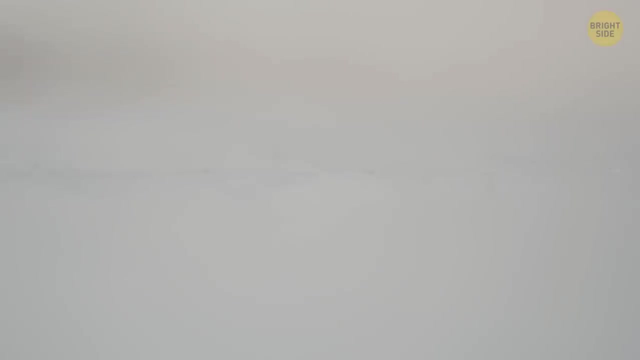 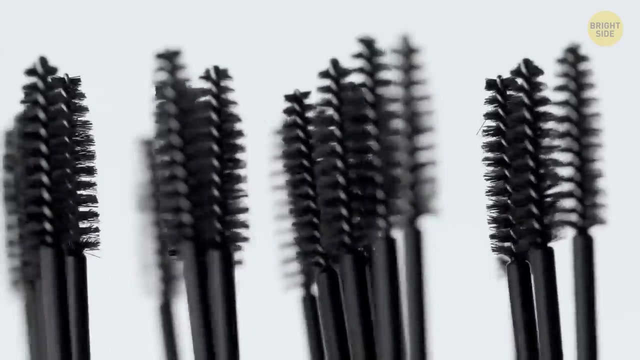 There's an easy way to check if your mascara is still good enough to use. If you don't hear a popping noise when you take the brush out, you may very well need to go get yourself a new mascara tube. So let's get started. 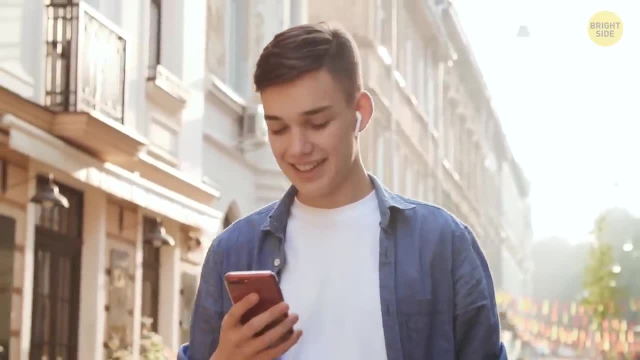 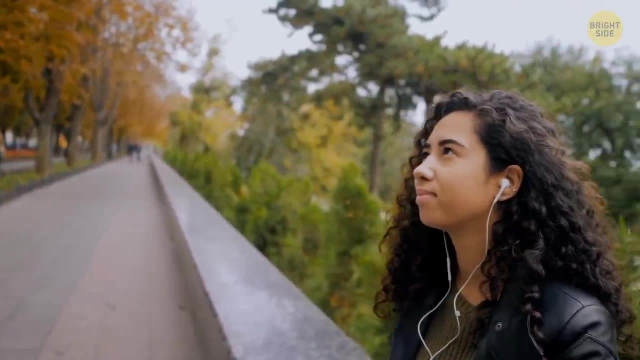 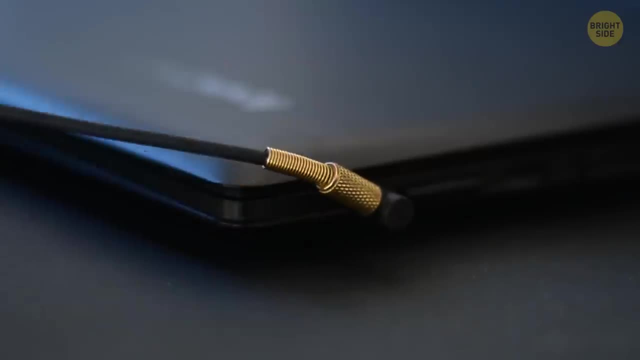 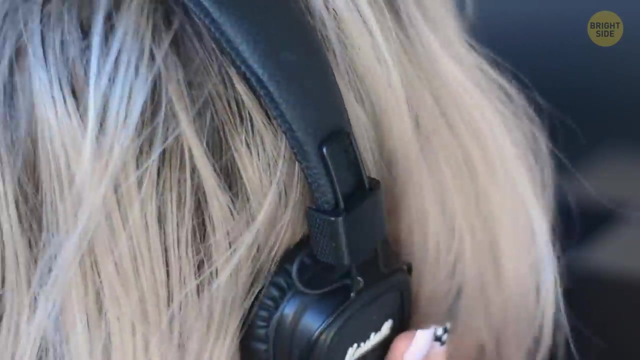 They aren't there just to make them fit when you plug them into your phone or laptop. Made out of a special insulating material, these bands are meant to guard the wires when sound is being transmitted. Based on the number of bands, you can figure out which end goes where. 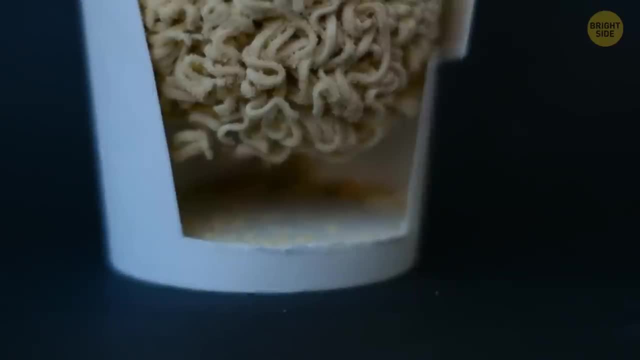 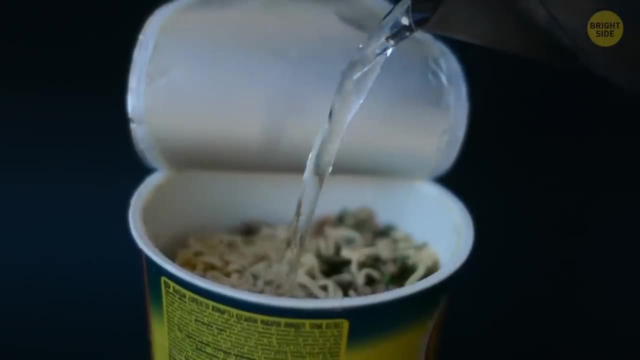 Some empty speakers. some empty space under noodles in a cup doesn't mean the company producing them wants to cheat you out of a full portion. No, no, It's a manner of keeping the noodles intact during their transportation. It also helps with the circulation of hot water. 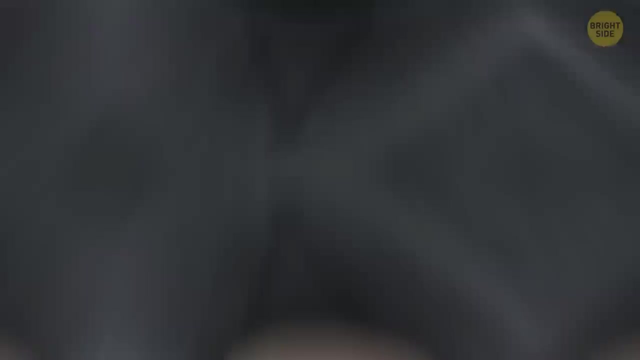 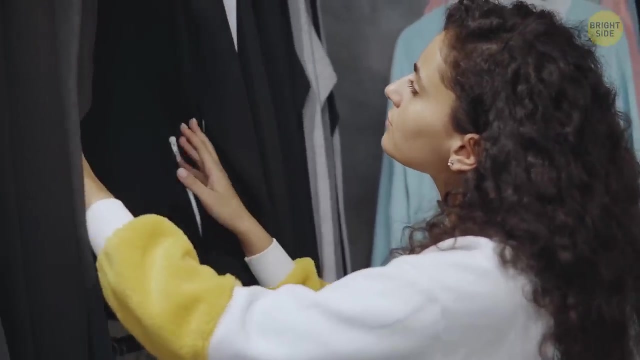 that is poured over the products before you can enjoy them. The V-shaped neckline was initially designed to serve a bunch of objectives. First, as a way of prolonging the life of the garment. that would maintain its shape over the years. It's also there to fit your head through the shirt. 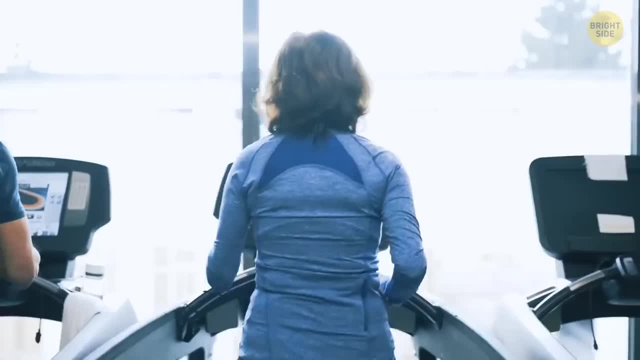 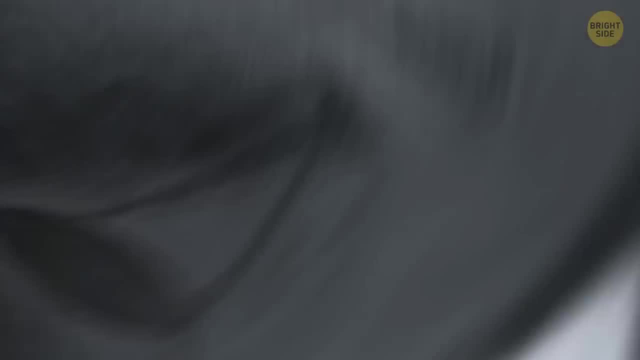 in case it needs some stretching. This way, it ensures a snugger grip around the neck. Lastly, it helps absorb sweat, in case you're wearing the shirt while exercising. Now it's not necessarily a custom anymore, but you may have stumbled upon a dinner jacket. 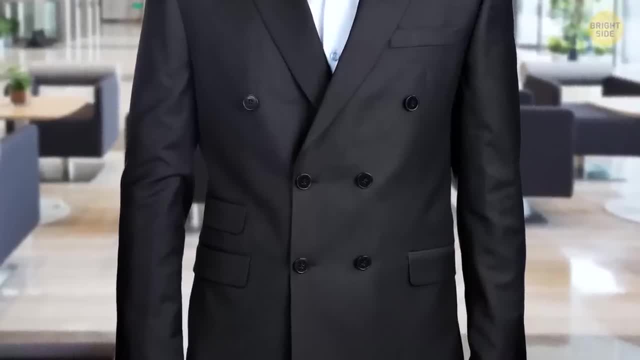 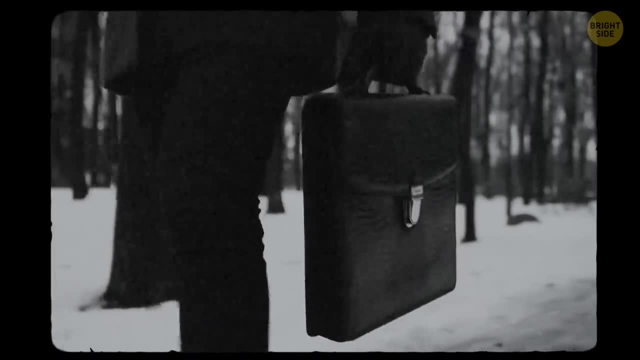 with an additional mysterious pocket on the right side. Turns out, this pocket was used by men to easily reach their train tickets, since most of them had to travel to work every day. It helped them keep their jacket buttoned up, but also benefited from the use of a pocket. 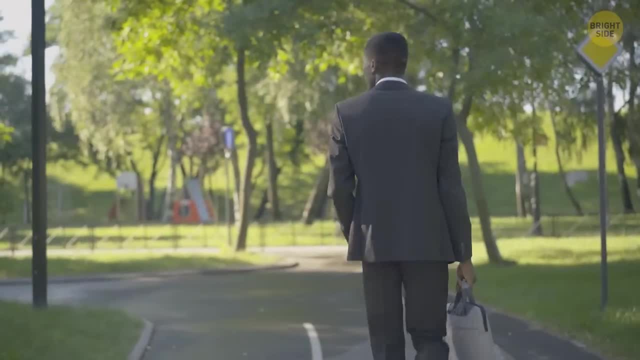 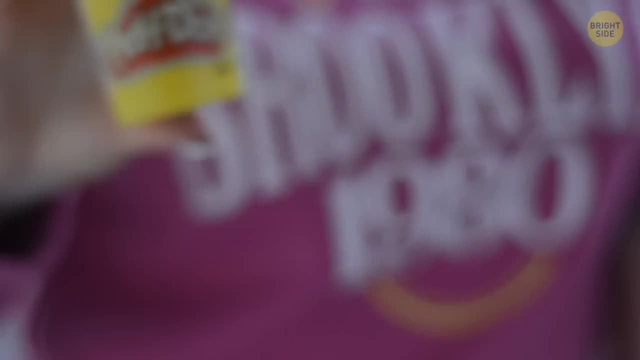 Now it's only added as a decoration and it doesn't serve an actual purpose anymore. Speaking of things we don't use these days, or at least for their initial purpose, did you know Play-Doh was originally a cleaning product? In the 1920s, the market was in need of a product. 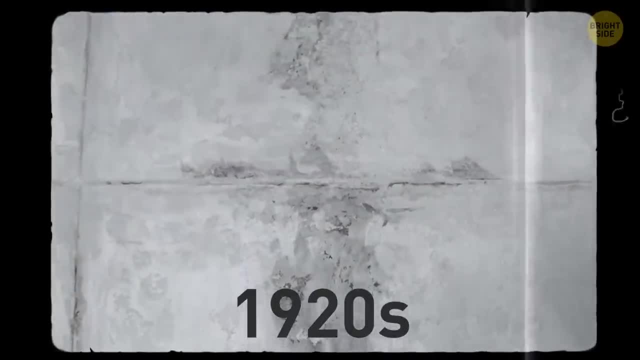 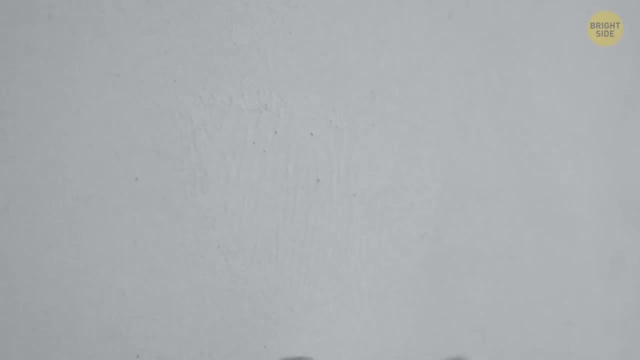 that could help them wipe the wallpapered areas around coal-burning furnaces. The recipe for what we now know as Play-Doh was thus invented. It was made of a plastic manufactured in white only and was supposed to clean wallpaper by being rolled back and forth over the dirt. 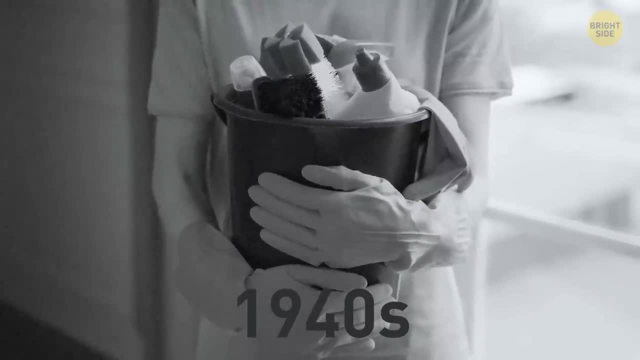 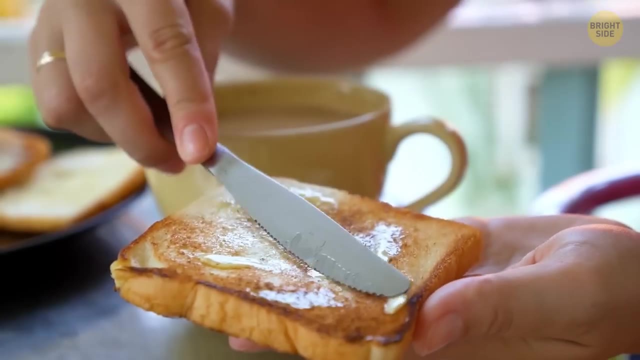 It was only later, in the 1940s, that new products for cleaning wallpaper were brought up, and Play-Doh was redirected toward another area of the market. Now, while I enjoy a nice piece of toast for breakfast, isn't it pesky to have to clean out the toaster? 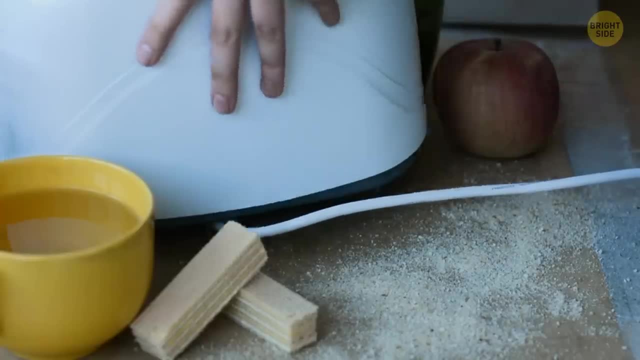 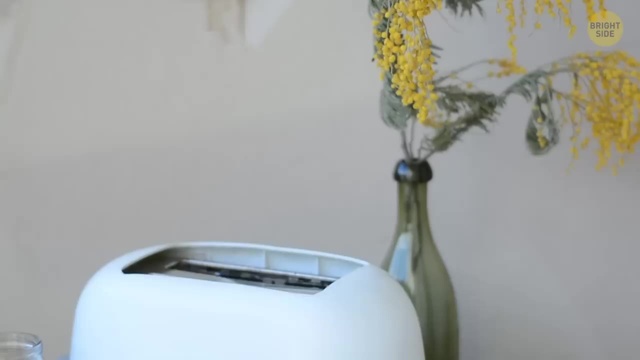 Well, not anymore, since I recently found out that toasters have a slide or a panel at the bottom that helps get rid of all those annoying breadcrumbs easily. Now, there used to be a time when you could only have access to video games. 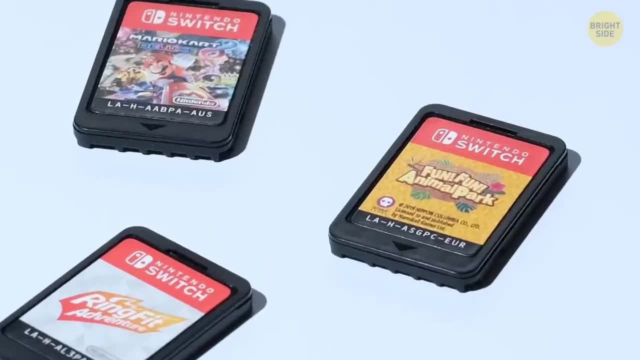 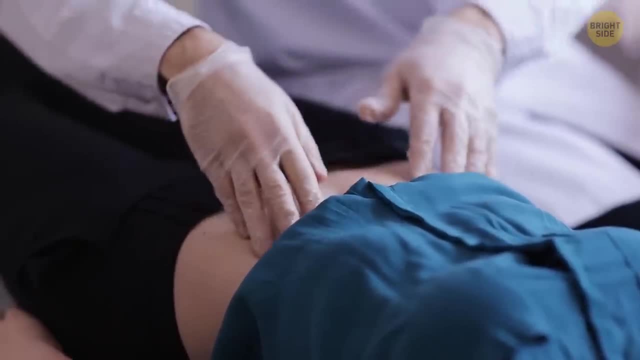 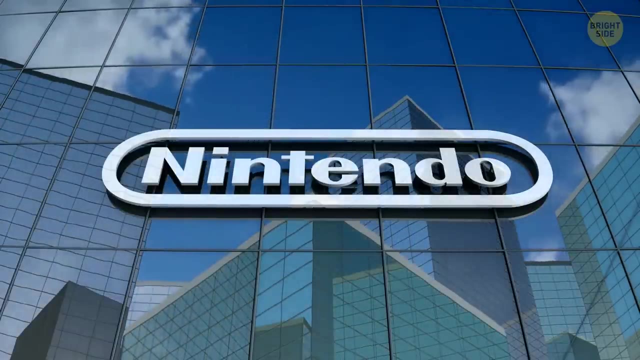 by inserting cartridges in your console of choice. These tiny objects gave many doctors a lot of headaches. People soon started popping up in hospitals after swallowing small game cartridges, especially the younger generation. Nintendo, the company that manufactures the majority of these devices, had to come up with a new method for cleaning up the mess. 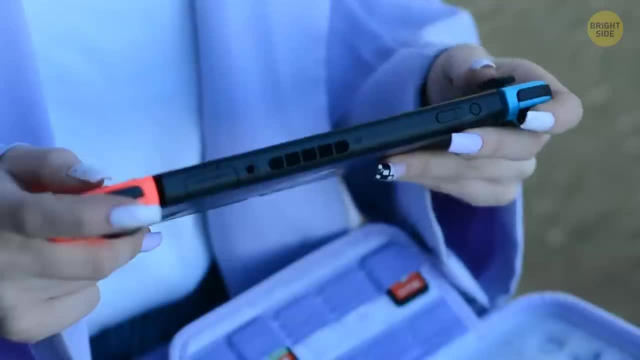 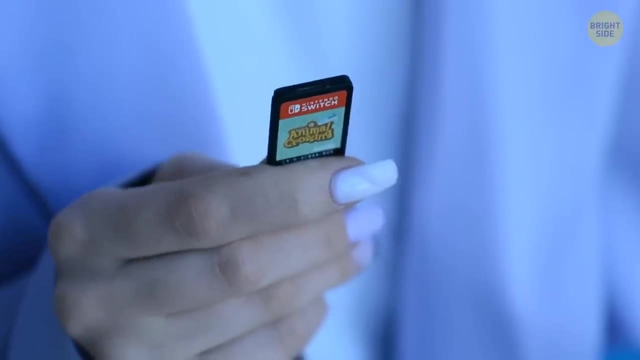 had to come up with a creative solution to prevent these accidents. So these days, Nintendo Switch cartridges are purposely coated with specific chemicals that can leave a really bad, bitter taste in the mouth. Not that I'd, you know, recommend you ever try and taste for yourself.